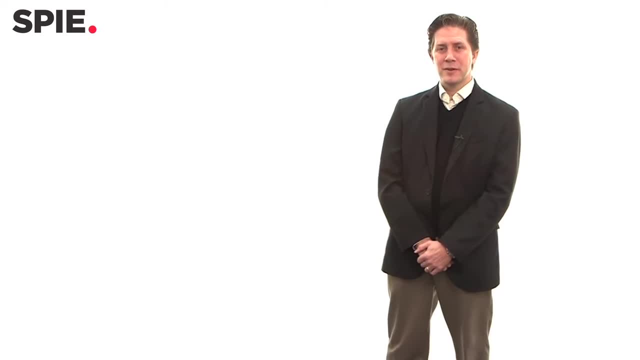 Science and Technology at Illinois. In my lab we develop novel optical biomedical imaging technologies and then apply them to solving problems in biology and medicine, And in particular we translate technologies from the bench to the bedside, but also then from the bedside to making an impact on clinical medicine. I think we've all heard of the phrase from: 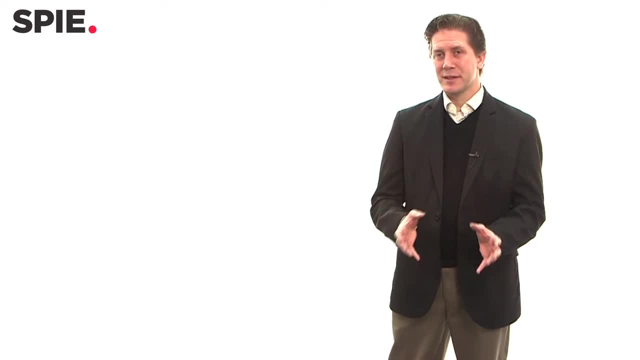 bench to bedside, and this is where we take new discoveries that are discovered in the lab and we translate those into applications for humans and perhaps in clinical medicine. But I feel that that's really important. We're only halfway there, So it's important to translate to the patient, but then we also 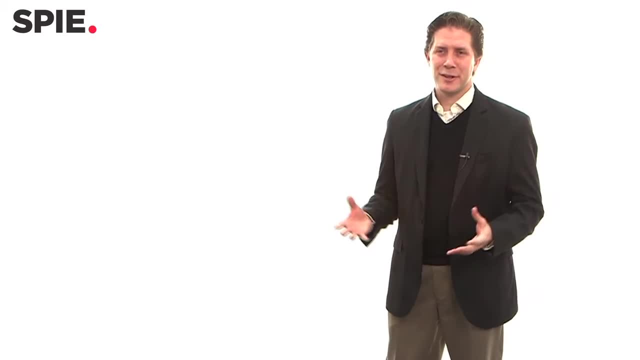 have to then move from the patient to the population, And so I like to call that transformational medicine and research where we can take our ideas but really change the standard of care or really impact our health and society in that way. So a lot of the technologies that 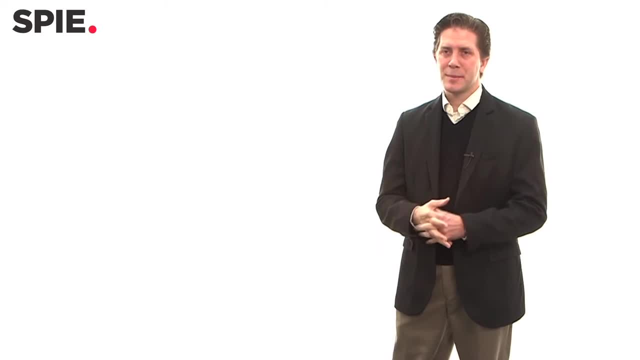 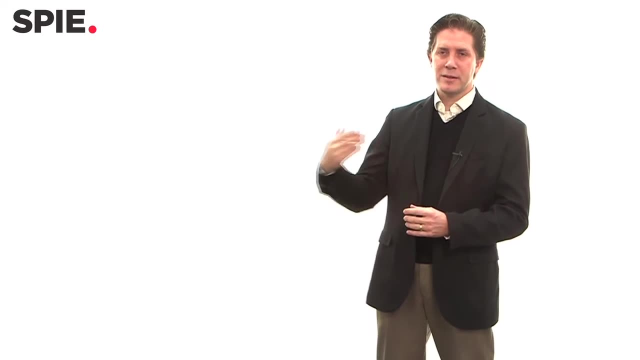 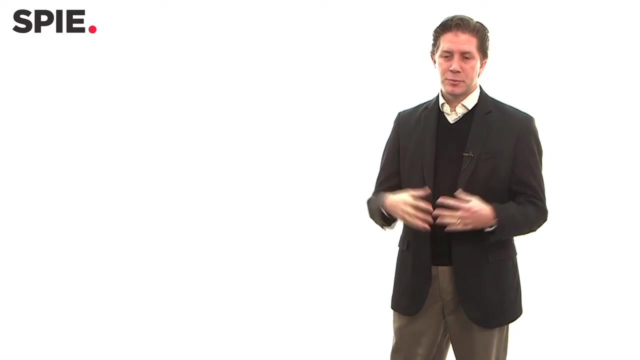 are developed in my lab and many other places. many other labs around the world, I believe, are focused in the same way. I think that's a really important area And it need to be, because we need to be thinking how we can really change the world. We can do that as an academic institution to bring 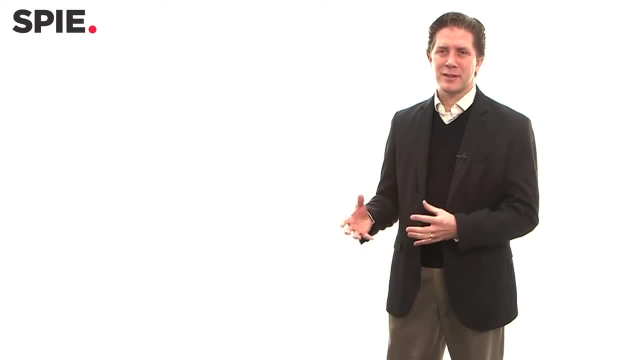 our ideas to the patient, translate those ideas. But we really need to partner with industry if we're going to transform things and change the practice of care. And the reason for that is because, obviously, we have to disseminate our ideas, We have to be able to develop safe 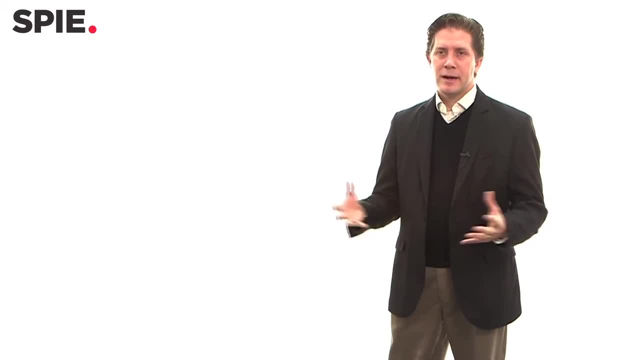 and approved technologies that can then be used to develop a new kind of care, And that's one of the things that we're really interested in, And we're really looking at the potential of the research that we do. So in order to do that, we're going to need to have a lot of research that's focused around care, And we're looking at what we're going to do to be able to do this in a way that's really important to the patient And that's going to be a lot of our research and research that's going to be able to be investigated at multi-institutional trials, and to be able 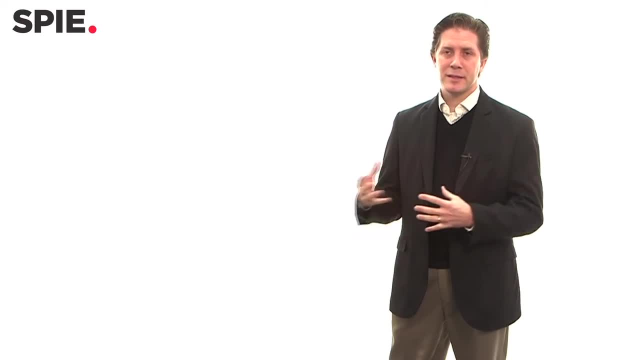 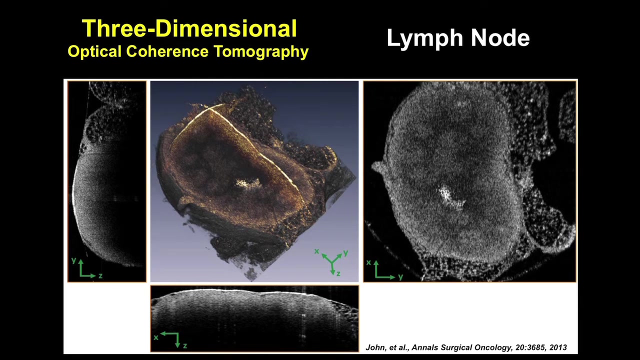 to apply to larger patient studies. So teaming up academic and industry-type partnerships, I think, are going to be essential for doing that. One of the focus areas for my group has been in using optical technologies to diagnose and help in the treatment of breast cancer, And this has been work that's been going on. 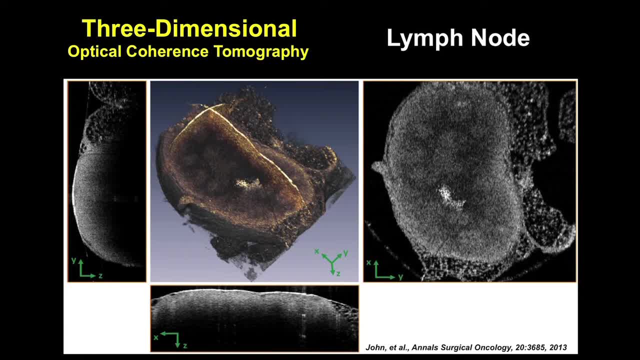 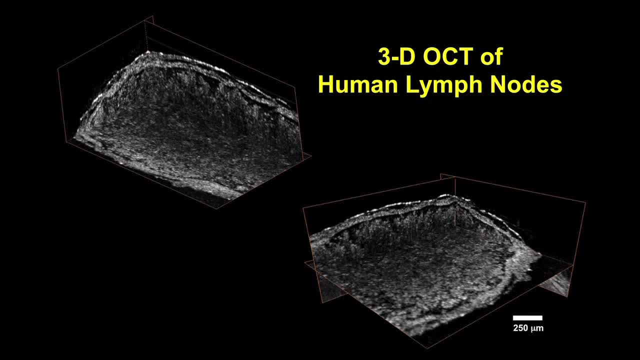 probably for over 10 years now in my lab, again starting at the bench level, where we're using optical techniques like opto- ط�ل coherence tomography to be able to identify breast cancer in resected specimens, but then begin to 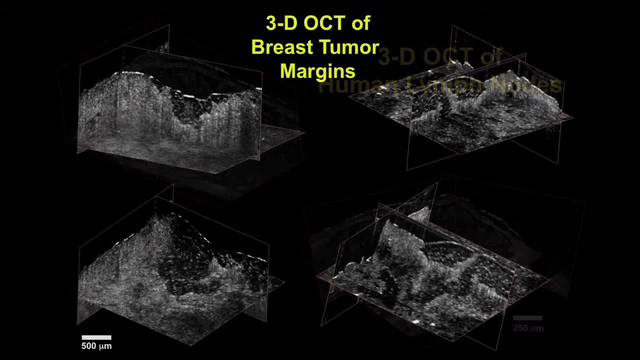 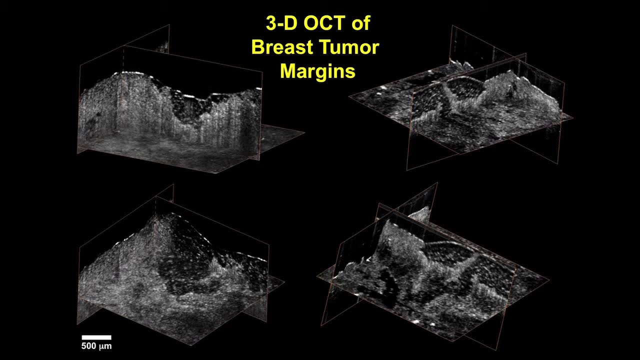 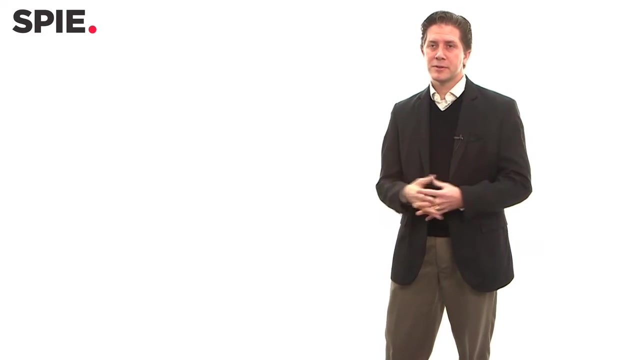 translate this. So we develop portable systems, including handheld probes, where we can take our new systems into the operating room and be able to look at resected tissue specimens. And even now, today we're using advanced systems that can do imaging in vivo, so in the tumor cavity, And we 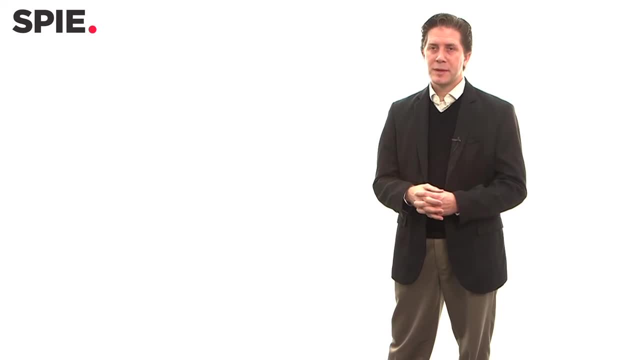 have systems that the surgeon would use now a probe, to be able to examine the tumor cavity and to be able to determine if there's any residual tumor cells left behind after the the tumor was removed. And this is important because over 30% of breast cancer surgeries actually result in reoperations. So the tumor is removed, the patient goes home, the tumor specimen is examined by pathologists in the path lab several days later oftentimes, And it's only then that's discovered, when they had a chance to microscopically examine the tissue. 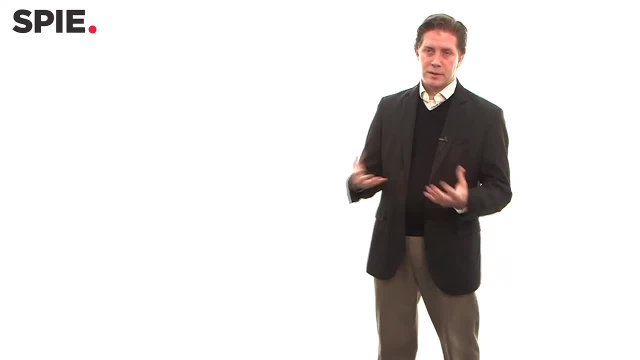 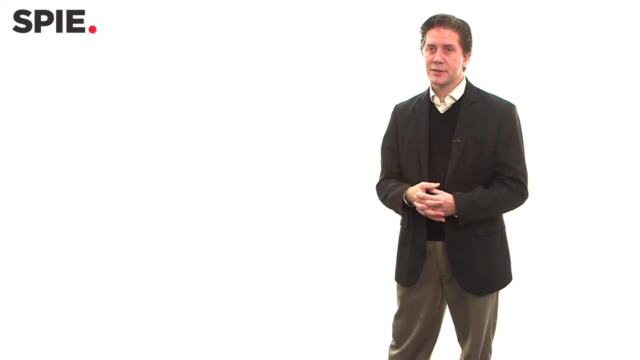 that they have to be able to bring the patient back to remove more tissue. So techniques like optical coherence tomography allow us to be able to give that microscopic view to the surgeon in real time, So he or she can then interact and respond to that information immediately. So 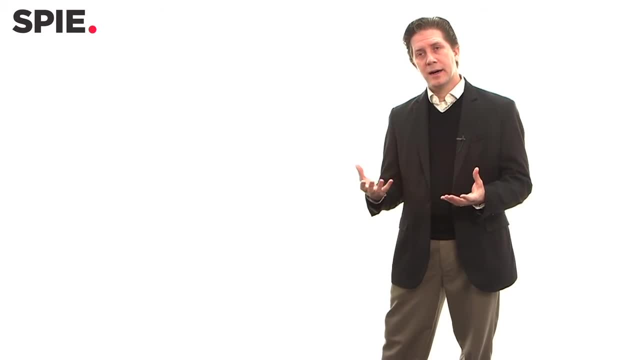 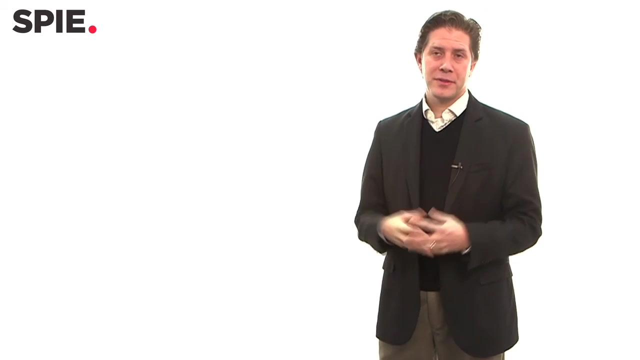 this is this technology. as I said, in order to be disseminated more broadly, we started a small startup company, Diagnostic Photonics, which took this technology, is building commercial systems and is now involved in larger multi-institutional trials, Along with the use of optical coherence tomography for looking at breast. 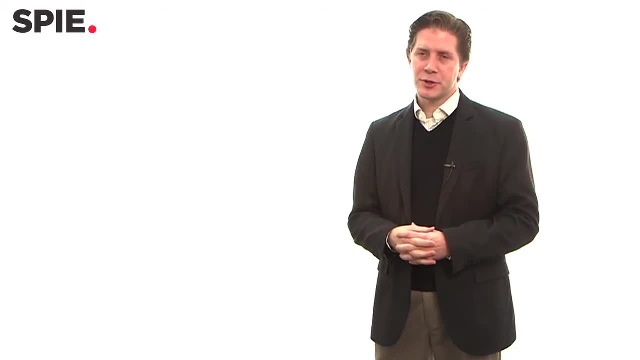 tissue- one of the things that we know, and by observing what surgeons currently do, they oftentimes will feel around the tumor cavity. they'll palpate to determine if there's any residual tissue left in there that may be left behind. Well, this is an indication that there are. 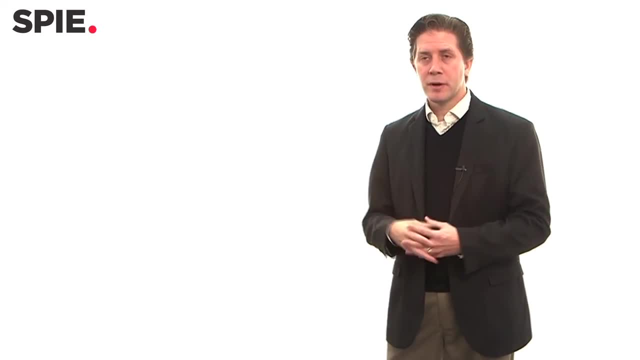 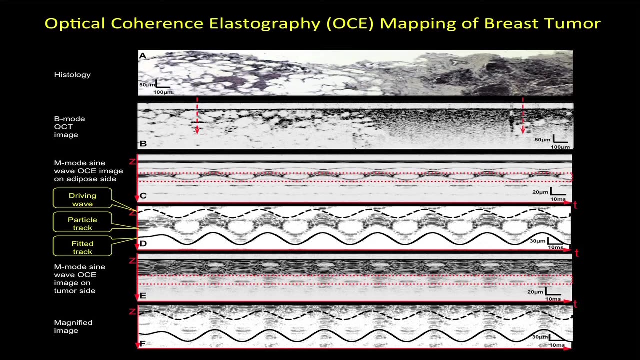 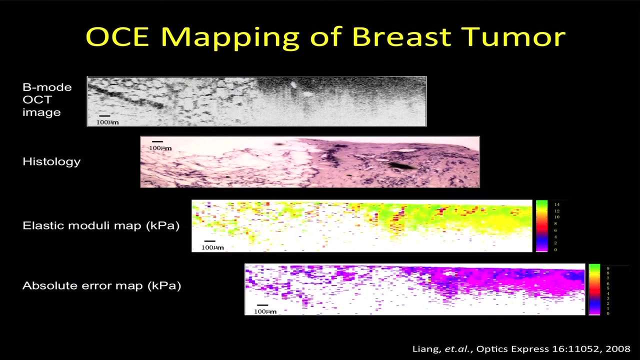 mechanical differences in the tissue that could suggest disease. Well, one of the ways that we can then develop optical imaging techniques to look at these biomechanical properties is through a technique we call optical coherence elastography. Now, this essentially uses an OCT platform.